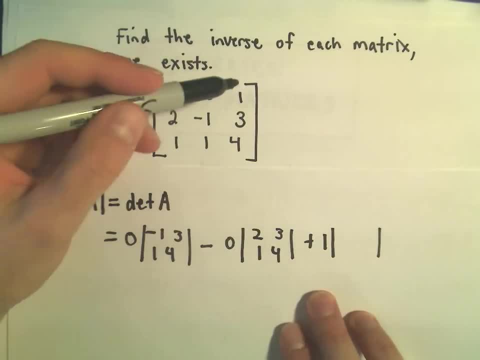 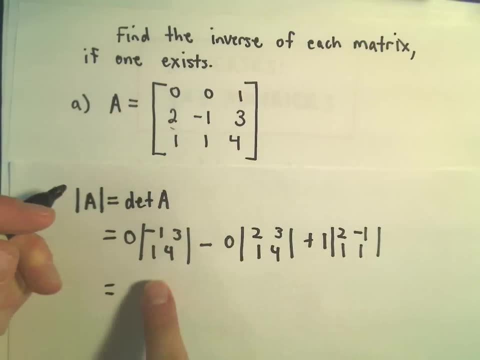 And then we'll add. We'll add 1 times. we'll have to take the determinant of 2, negative 1, and 1, 1.. Well, the first one's 0, the second one's going to be 0.. 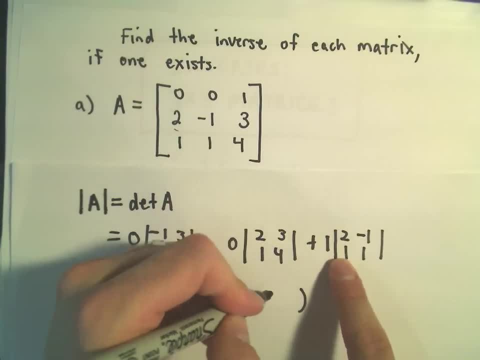 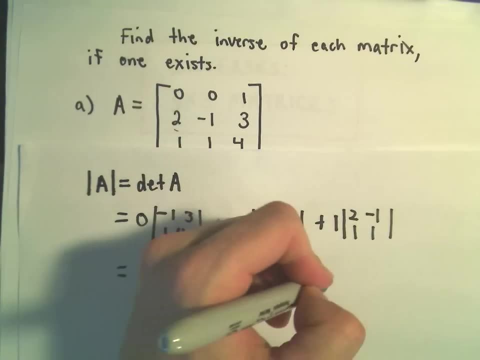 Then it looks like we have 1 times. let's see, we'll get 2 times 1,, which is 2,, minus 1 times negative 1, which will be plus 1.. So it looks like we'll get 1 times 3, or we'll get the determinant to be 3.. 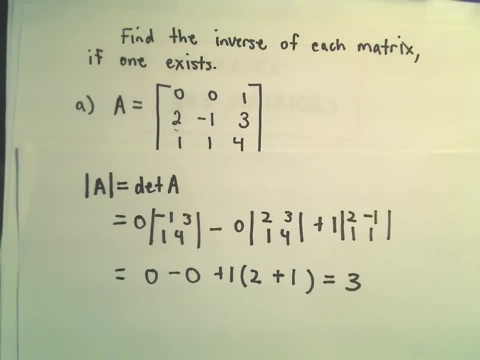 Okay, so that's one thing that's going to be. Uh, We'll have to use that here in a little bit. The next thing I'm going to do is go about finding I'm going to basically use the cofactors. So the way we do that is. 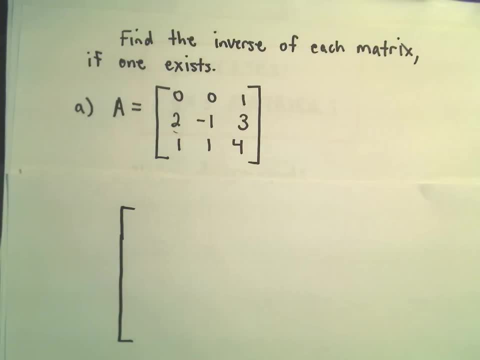 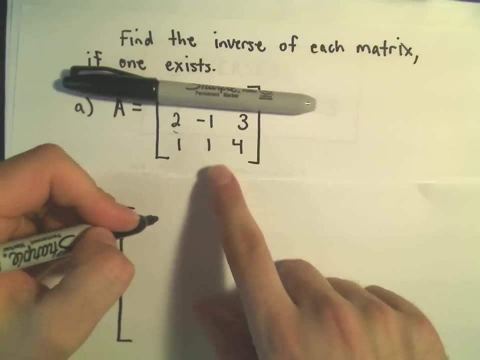 Basically I look at the first. If I cover up the first row and the first column, I'm going to be left with the numbers negative 1,, 3,, 1, and 4.. So that's what's going to. 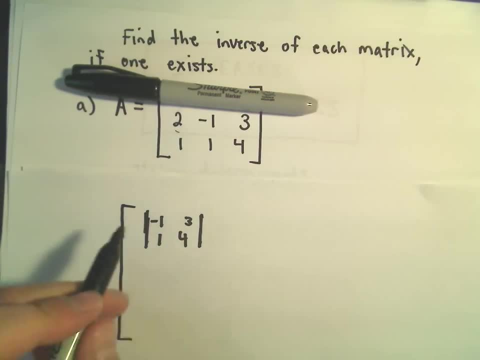 I'm going to calculate the determinant of that. I'm going to have to fill in some signs here in a second too, so I'll get to that in just a moment. Next, if we cover up the first row and the second column, it looks like we're going to be left with 2,, 3,, 1, and 4.. 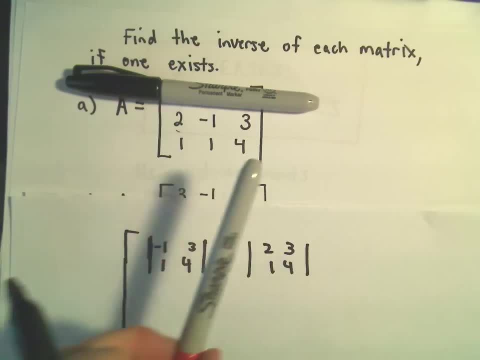 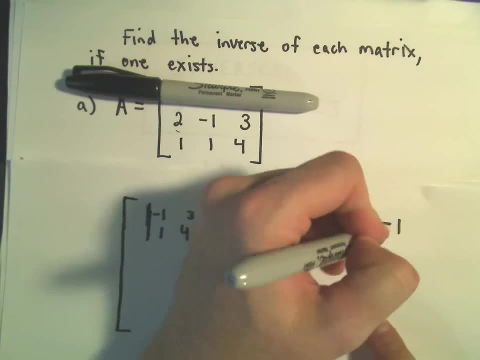 So 2,, 3,, 1, and 4.. And if we cover up the first row and the last column, we'll be left with the 2, negative, 1,, 1, and 1.. So 2, negative, 1,, 1, and 1.. 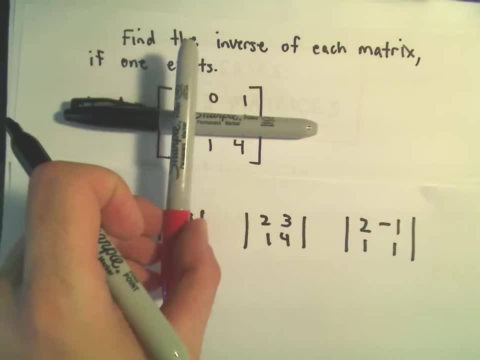 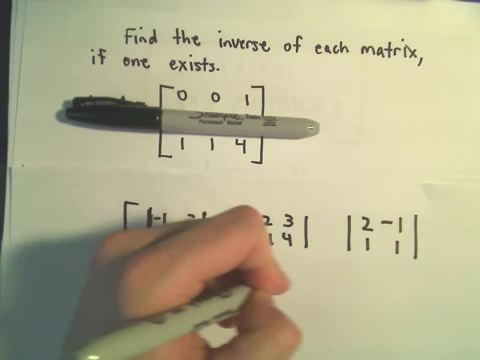 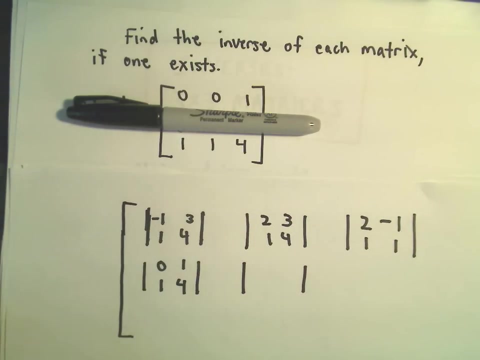 Next, if we cover up the second row and the first column, we'll be left with 0,, 1, and 1, 4.. So 0,, 1,, 1, and 4.. If we cover up the second row and the second column, we'll be left with- it looks like 0,, 1, and 1, and 4.. 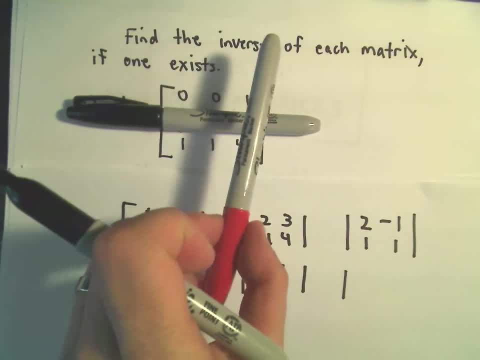 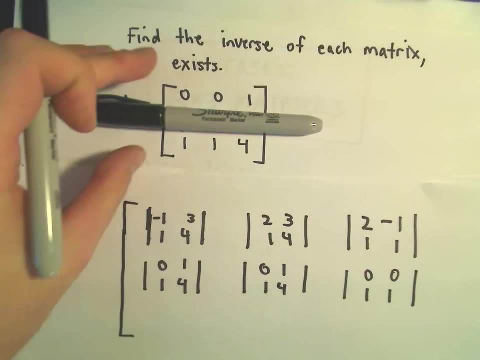 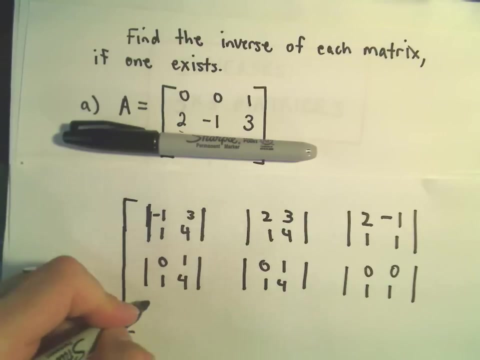 Let's see If we look at: If we cover up the second row and the third column, it looks like we'll have 0, 0, and 1, 1.. And lastly, if we cover up the third row and the first column, it looks like we'll be left with 0,, 1, negative 1, and 3.. 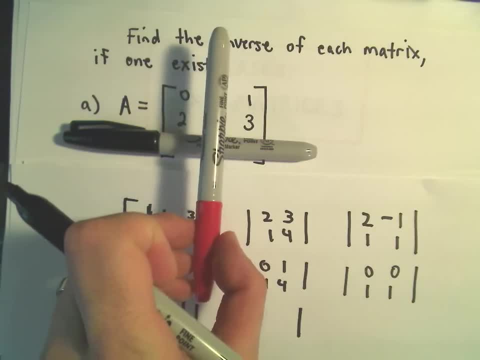 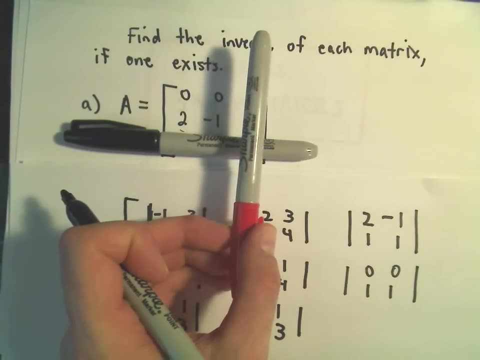 If we cover up the third row and the second column, we'll be left with 0,, 1,, 2,, 3.. And then, if we cover up the third row and the third column, we'll be left with 0,, 0,, 2,. 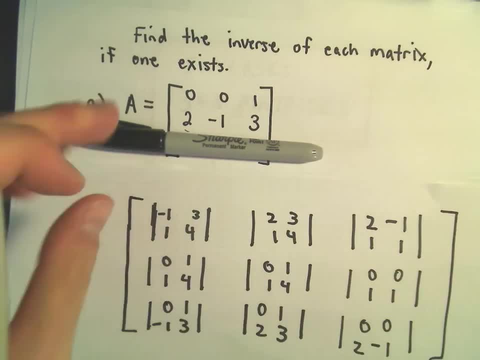 and 3.. And then, if we cover up the third row and the third column, we'll be left with 0,, 0,, 2,, 3, and negative 1.. So we still have to put our signs in here as well. 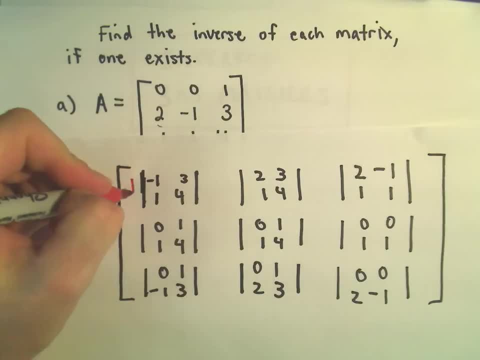 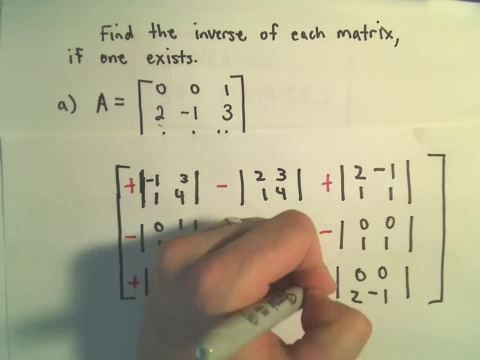 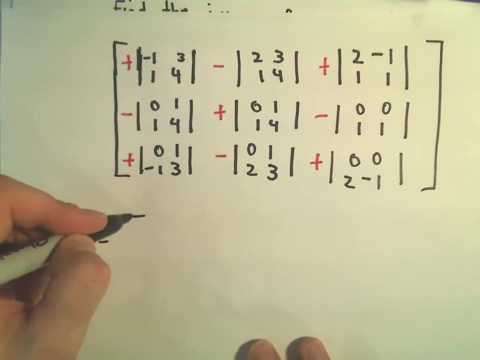 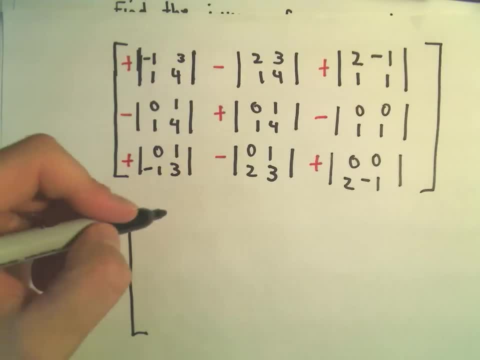 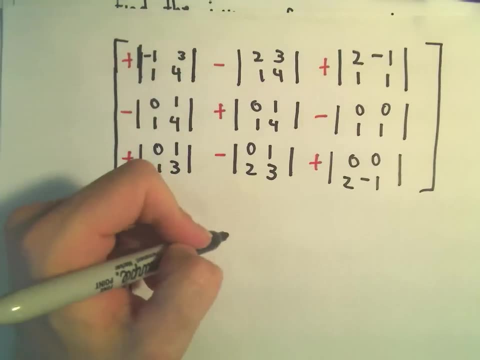 We would get negative 1.. It looks like we would get negative 4 minus That would be negative 7.. We would get 8 minus 3.. 8 minus 3 would be 5, but we have to use the minus sign out front, so we'll get negative 5.. 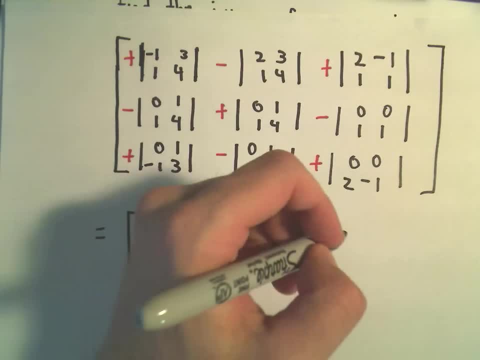 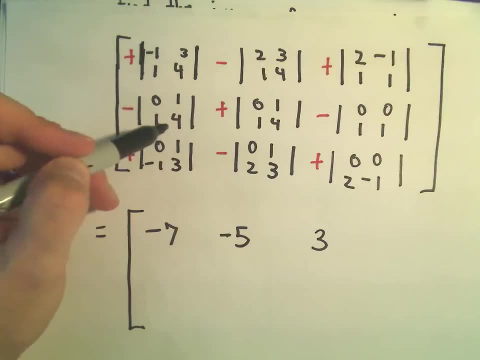 We'll get 2 minus negative 1, or 2 plus 1, which will be 3.. 0 times 4 is 0 minus 1, so we'll get a negative 1 for the determinant. but we have to multiply that by the negative, so we'll get a positive 1.. 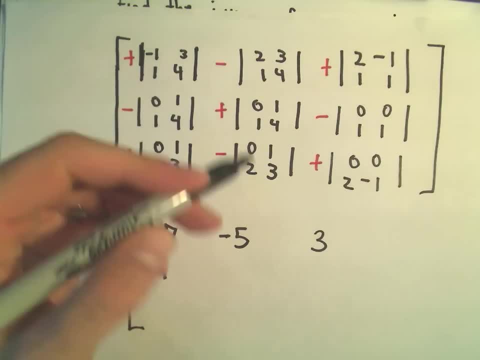 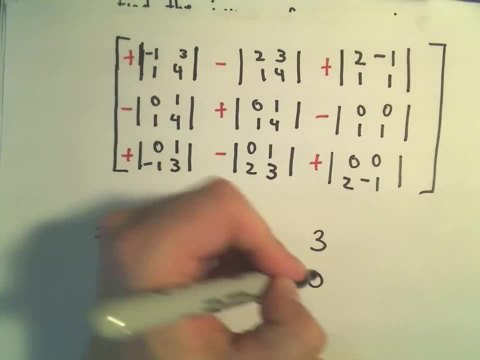 0 times 4 is 0 minus 1.. So we'll get a negative 1.. And then it looks like we'll just have 0 minus 0, so we'll get a 0 there. 0 times 3 is 0 minus negative 1.. 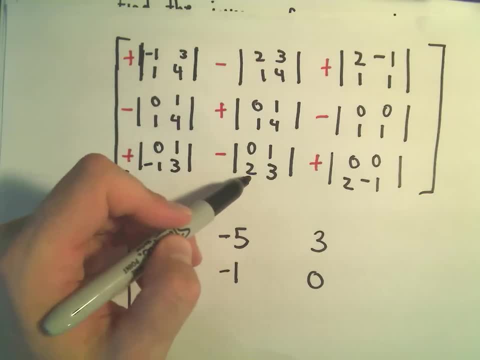 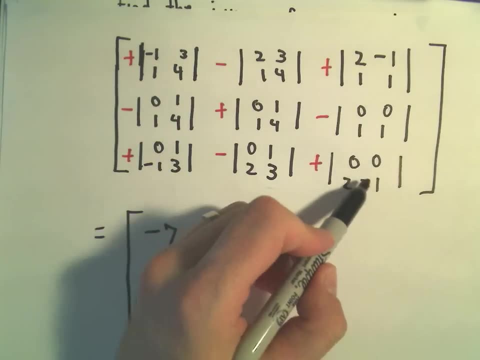 We'll give us a positive 1.. 0 times 3 is 0 minus 2, so we'll get a negative 2 for the determinant, but with the extra negative it'll switch back to positive 2.. 0 times negative: 1 is 0 minus 2 times 0 is 0.. 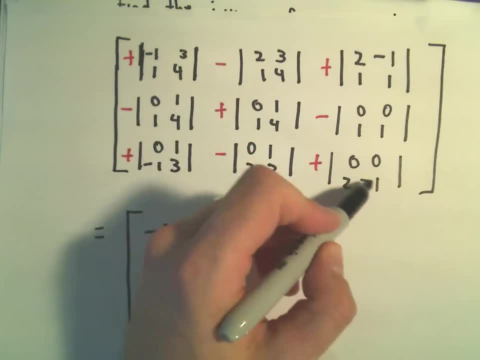 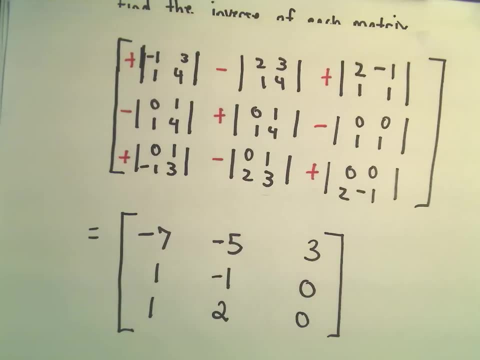 But this time we've got Well, it doesn't really matter, We've got a positive, but who cares? because we're getting 0 anyway, Okay. so the next thing we have to do is we're going to have to now do a little reflection. 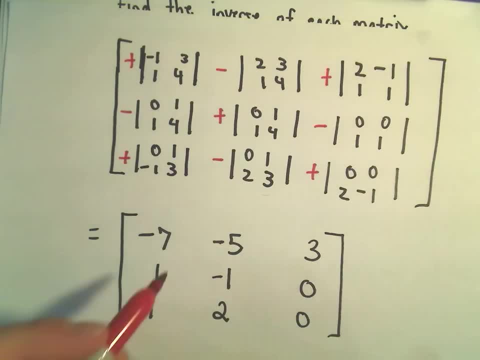 And what we do is we reflect things about the diagonal. So this is going to be the diagonal. Those numbers are going to stay right where they're at. Okay, so I'm not going to move those numbers at all. So let's see.